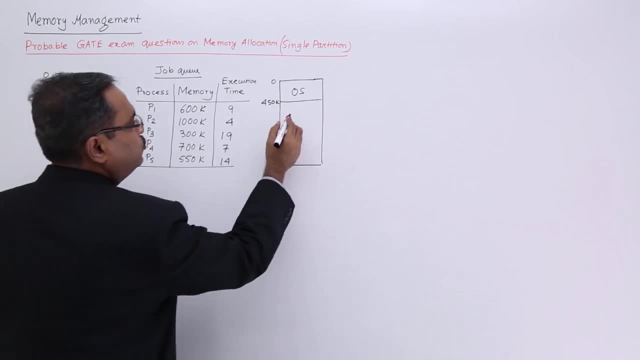 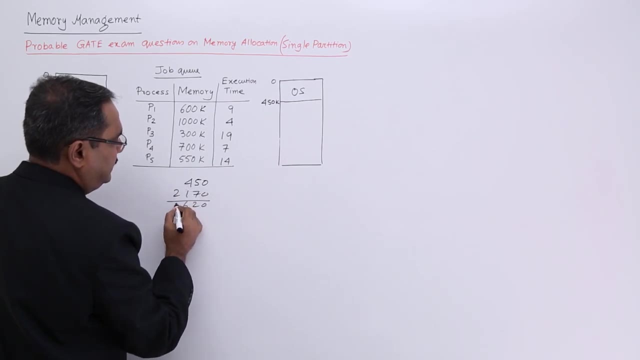 is 450 K plus 2170.. So 2170.. So 450 plus 2170.. It is quite obvious that this is the process. It is my 6 and it is my 2, ok, So very simple, I have just added. So 2620 is. 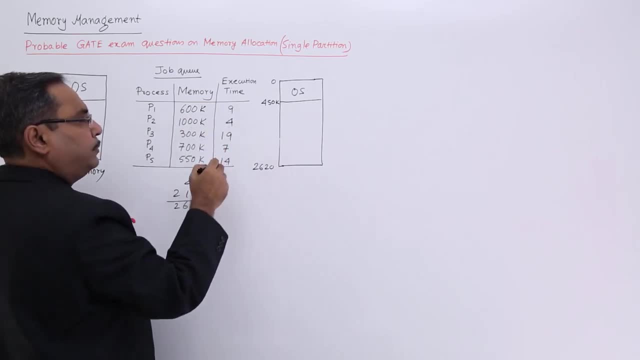 the total size. So let us suppose all of them are available. Let me go from P1 to P5 in this order. So at first P1 will get loaded. What is the size of P1? 600 K. So it will. 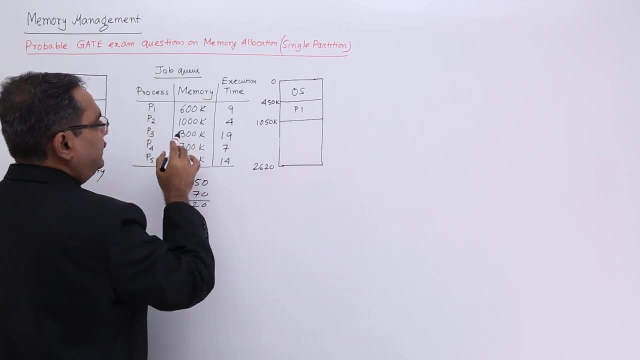 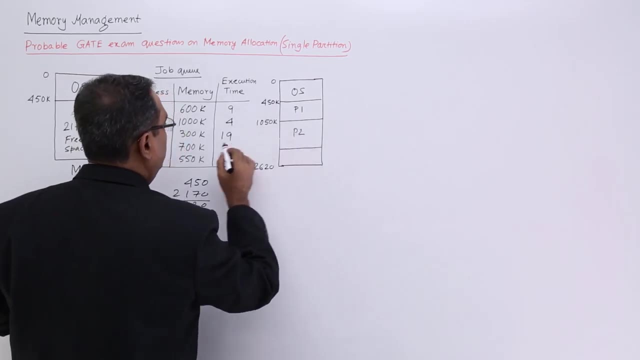 be 1050 K, Then P2 will get loaded. Will it get any chance? Yes, Spaces are there, So it will get loaded. What is the size? Size is 1000.. So that is 2050.. What is the size? 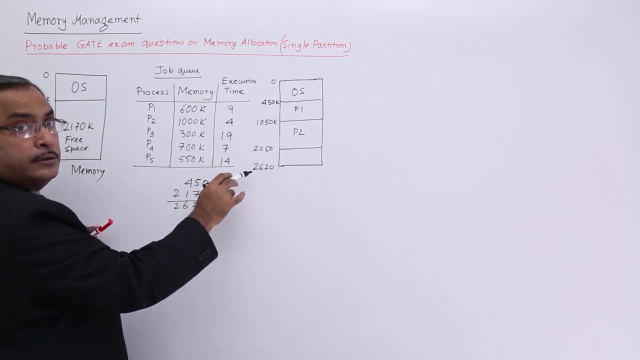 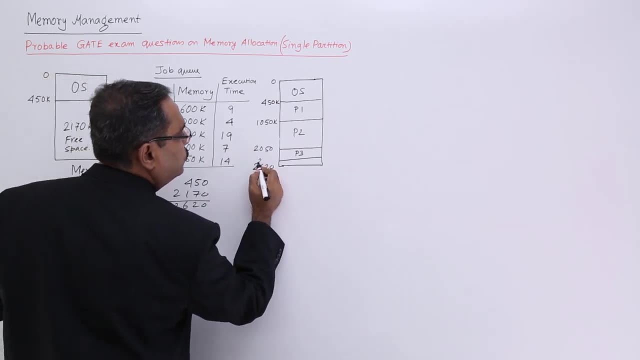 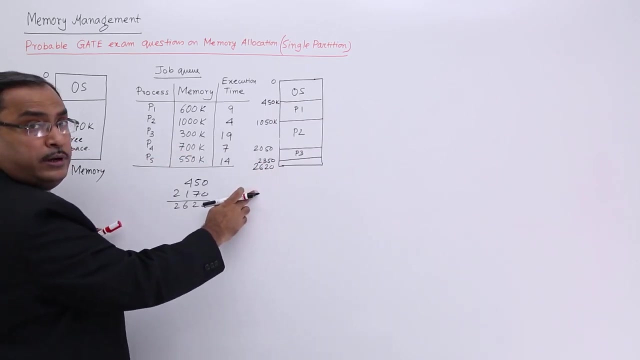 of P3? 300 K. Can it fit? Yes, it can fit. So now I shall go for P3.. So P3 is having the size of 300. So 2350.. What is the size of P4? P4 is 700.. What is the space in between? 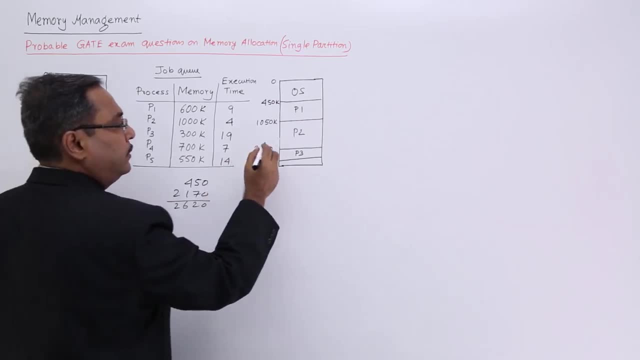 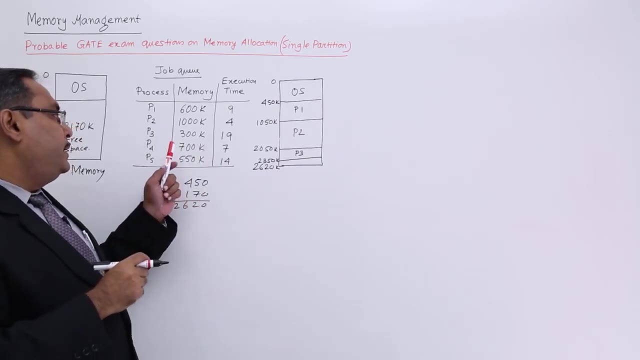 Lesser than 700 K, So it cannot be loaded there. All of them are loaded, So this is the number K. So P1, P2, P3 can get loaded at first. P4, P5 cannot be loaded, So now. 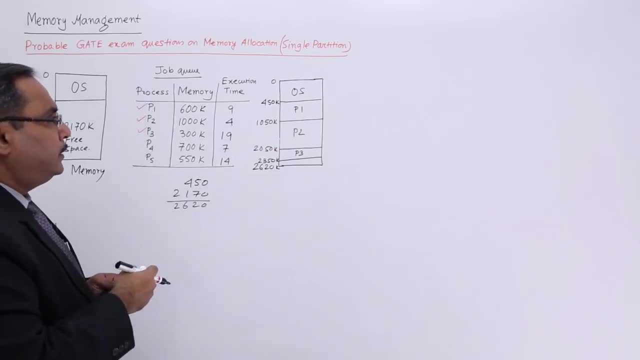 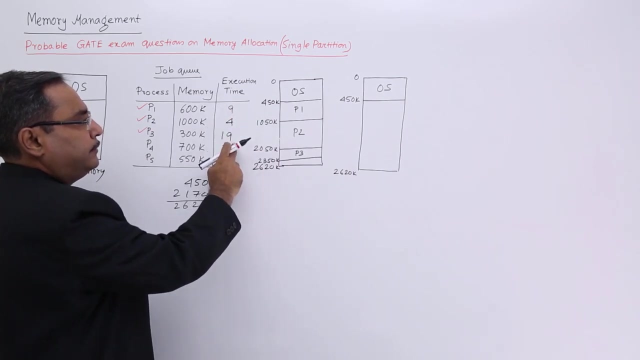 they have got loaded and they are executing Now. out of them, which one will get executed earlier, will complete earlier. The time is 9, 4, 19.. So 4 will get terminated earlier because the time is 9, 4, 19.. So the time is 9, 4, 19.. So 4 will get terminated earlier. 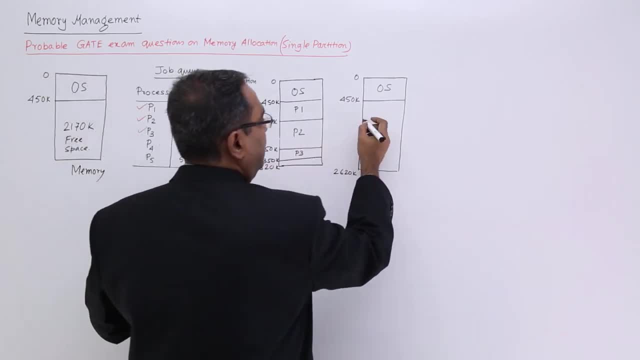 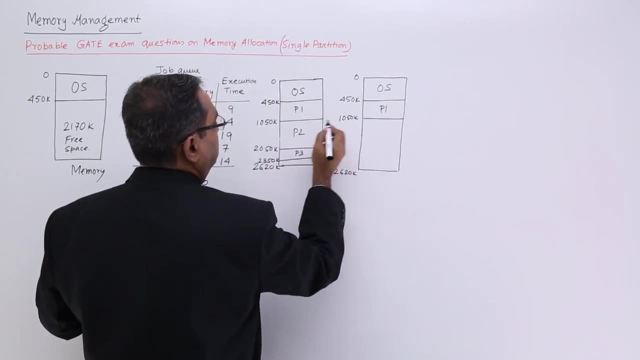 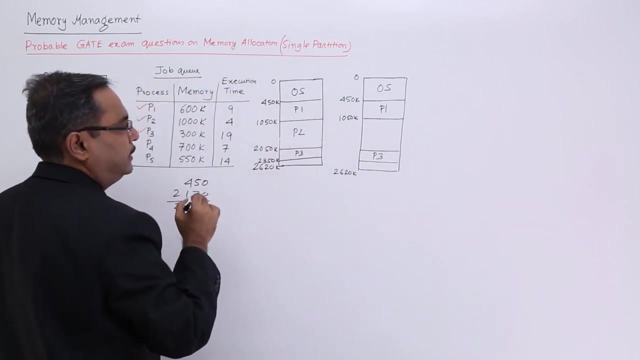 Because it is having the lesser execution time, So P1 will survive. P1 will be still there. P1 will be taking up to 1050 K. Then P3 will be there still And it is occupying memory space: 2050 K to 2350.. Because P3 is having the size of 300 K, So P2 has completed. 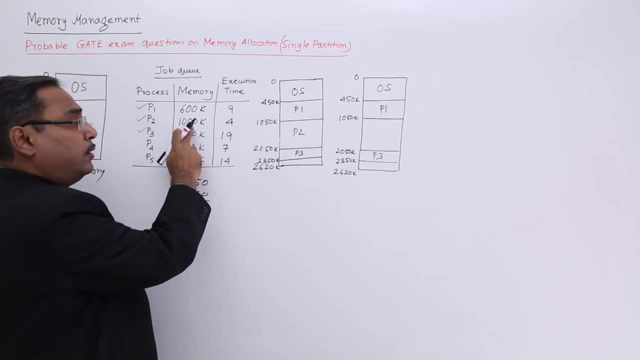 So the memory space occupied by the P2, what was the memory space? 1000 K? Is it 1000 K? Yes, So it has got freed. So now I shall go for P4.. So P4 will occupy 700 K, So I. 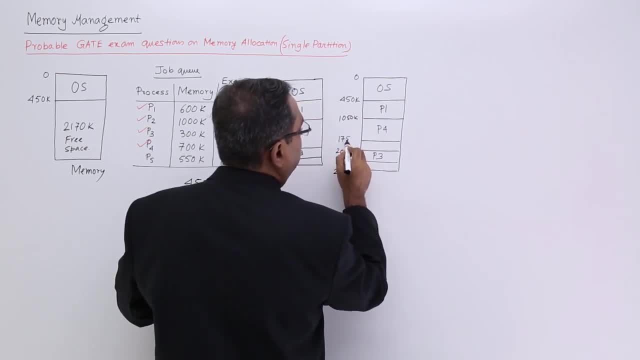 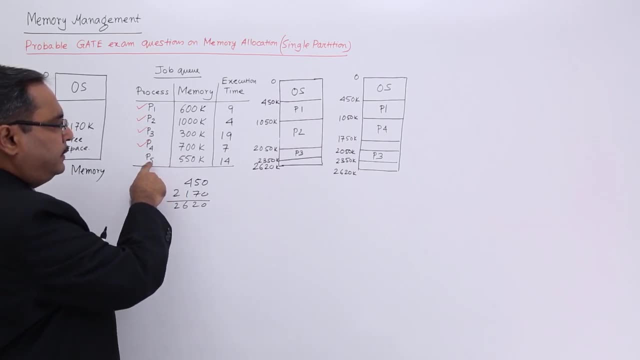 shall go for P4. So P4 will occupy 700 K, So that is a particular free space available. What is the size of P5? 550.. What is the size in between? Yes, What is the size in between? 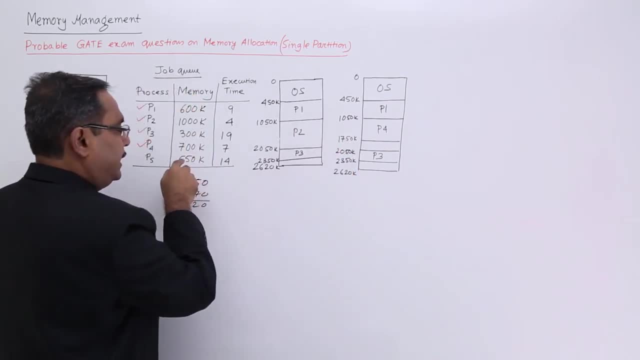 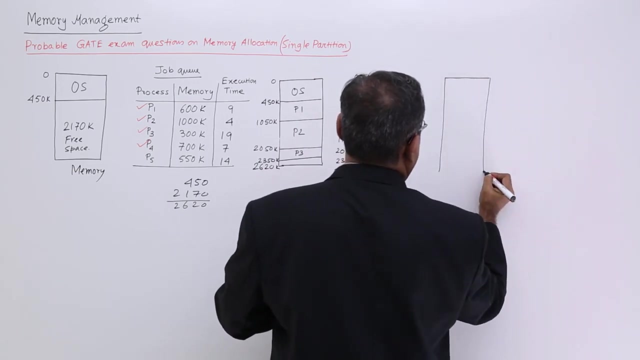 300 something. So the size is 300 K, which is lesser than this, And obviously the size is also lesser than this. Then I shall have to wait for that. So now P5 cannot be loaded In the next diagram. what will happen? So it is been done at the 0th instant and it 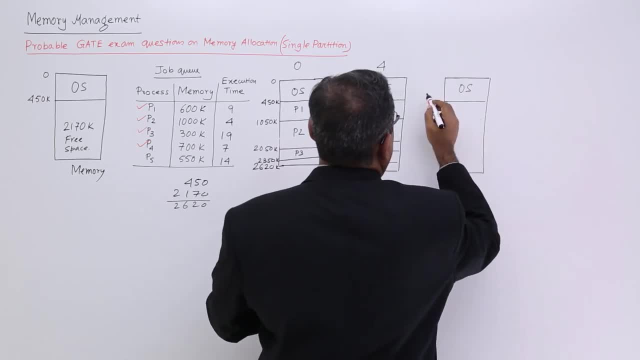 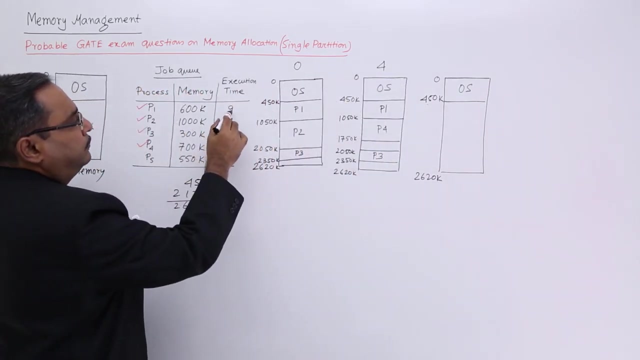 has been done at the fourth instant Because P2 was having that duration. There is a four unit of time And this is again a different sort of situation, So they can be loaded. So now it is 450 k and this processes are there and that is 2620 k. So now it has. 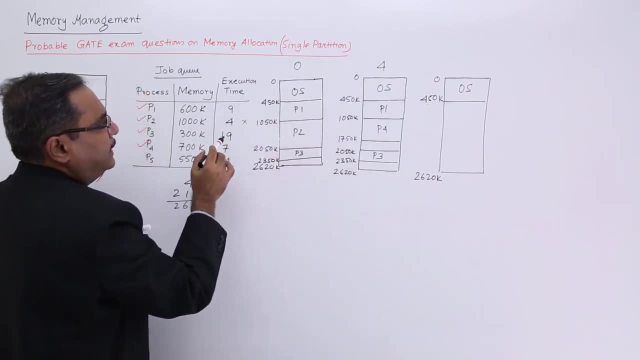 got completed after this. So what is the execution time now? Who will get terminated at first? So it is remaining with 5, it is remaining with 5, it is terminated. it is remaining with 15, it is remaining with 15 and P4,. P3 has just come. P3 has just come. 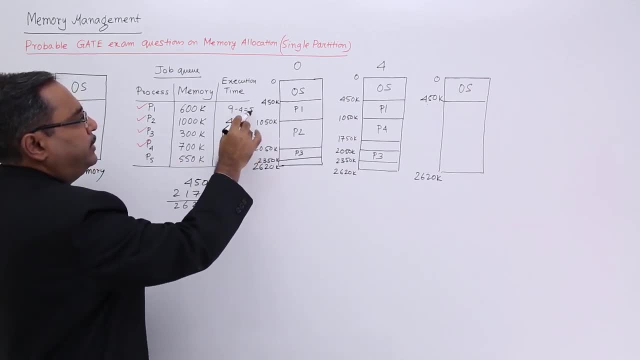 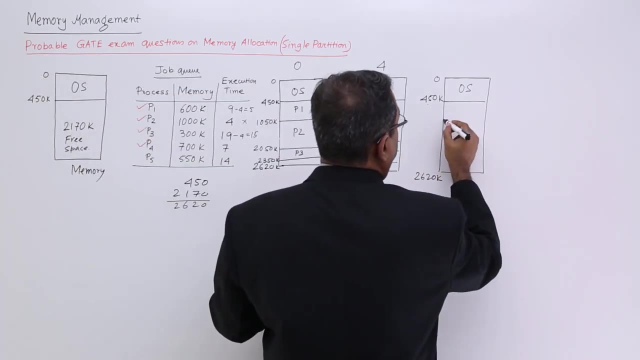 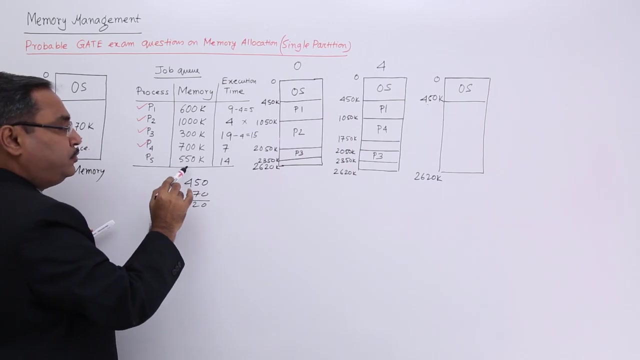 So this is a P3 has just arrived. Now who will get terminated at first? P1 will get terminated, So P1 will get terminated at first. So now, what is the size of P1? P1 is 600 k. What is the size of P5? 550 k, So that can be loaded. So now at the 9th, 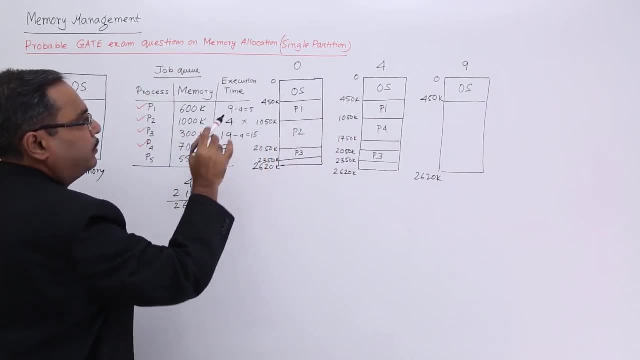 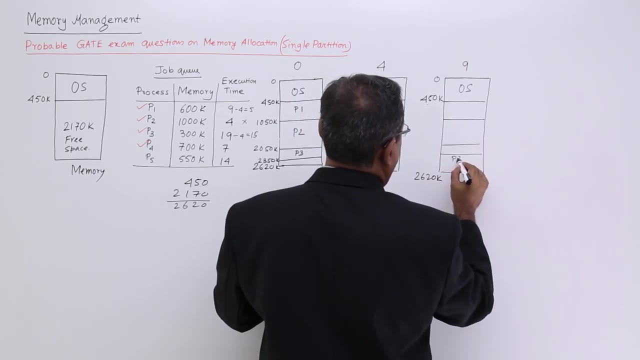 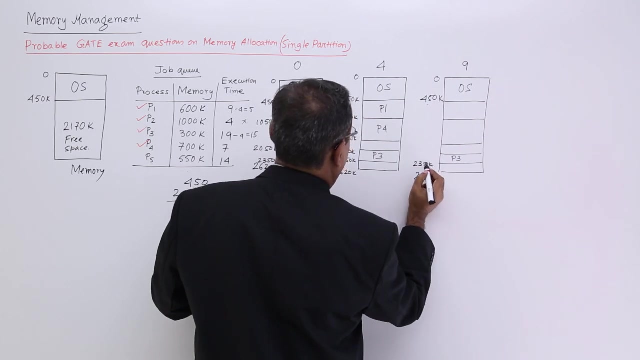 instant, at the 9th instant, because that is the execution time of P1, P1 will get terminated, So P4 will survive and P3 will survive. So here it will be 2350, as usual, This is a 2050. 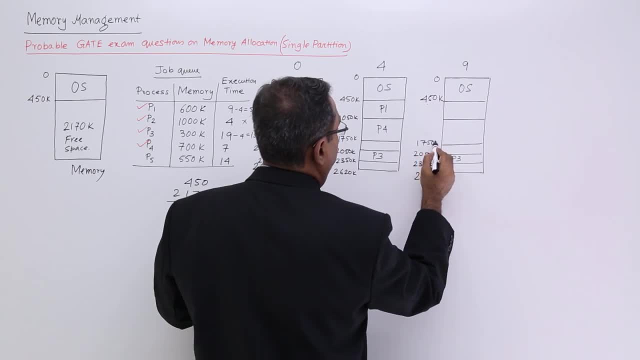 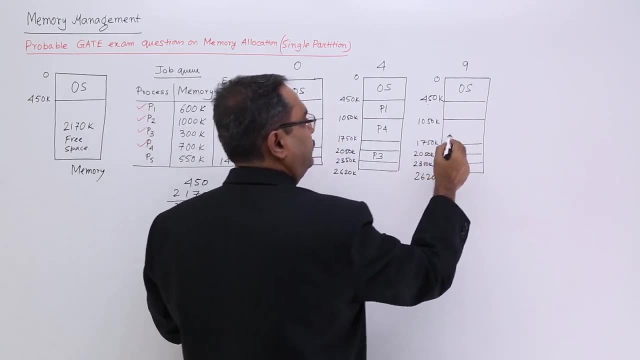 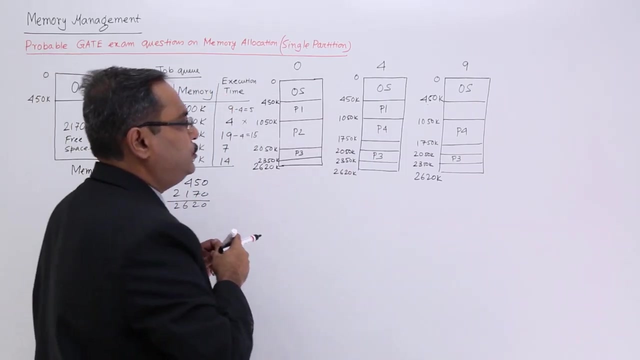 k as usual. It is 1750 k as usual. So that is 1050 k as usual for 2050 k. So this is P1, P4.. And now P5 will get loaded, So that is a 550.. So P5 will get loaded, P5. So